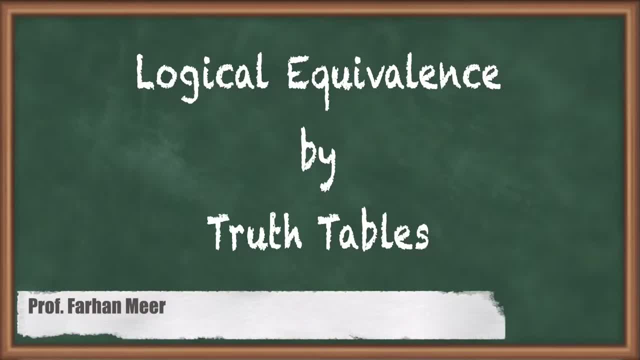 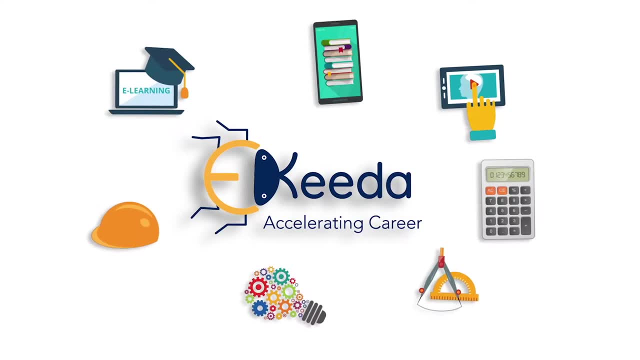 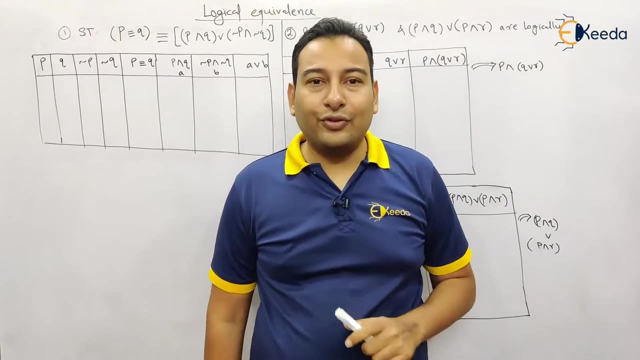 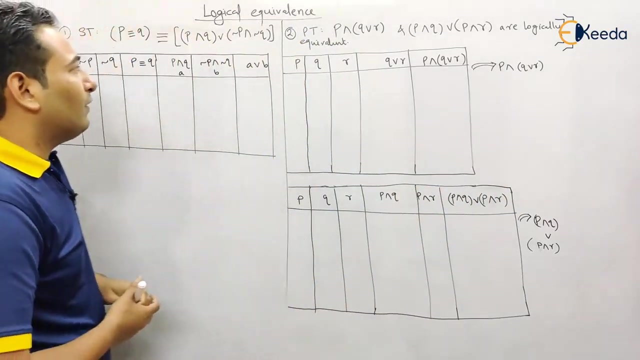 hello friends. in this video we'll talk about logical equivalence of two statements with examples. welcome back, friends. now let us discuss logical equivalence of two statements and we're going to solve these two examples are based on that, so let us start. first of all, we are showing logical equivalence. 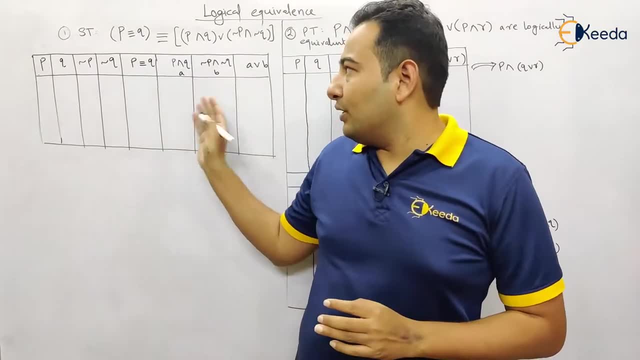 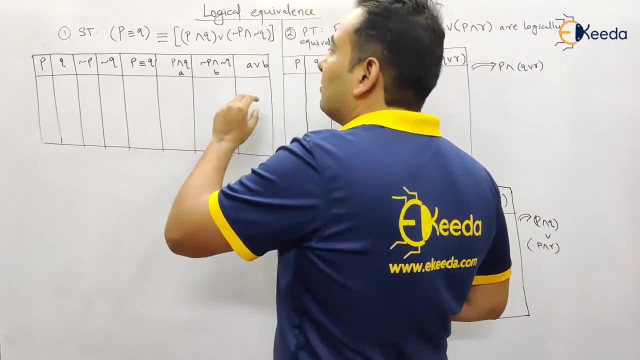 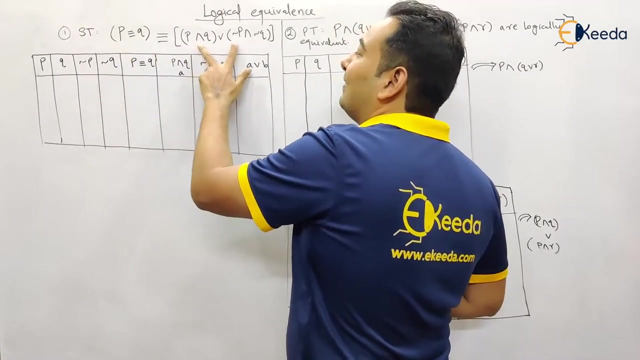 between the two statement by using root table method. so therefore, the tables are already made by me. now, just to save time, let us start now. what is the first question in the first problem? we need to show this is equivalent to this. so logic. we need to show the logical equivalence between this statement and this. 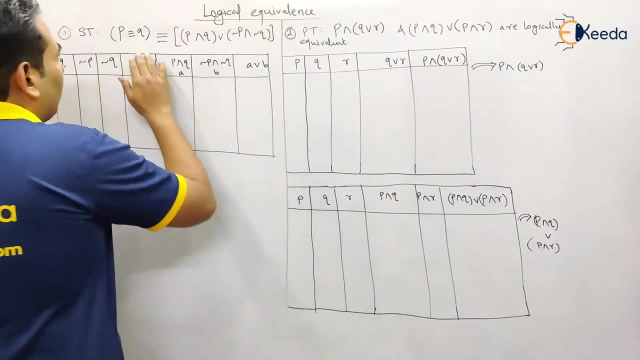 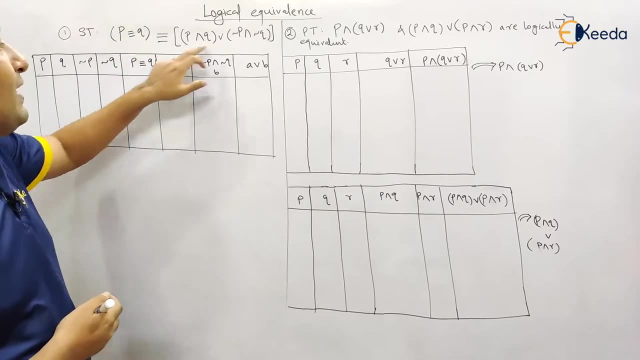 statement. so first of all, let us start, since, if you observe the entire statement, there are only two values, that is, P and Q. since there are two values, that is P and Q. since there are two values, that is, P and Q. since there are two values, P and Q, so there will be 2 raised to 2, that is, 4 combination. 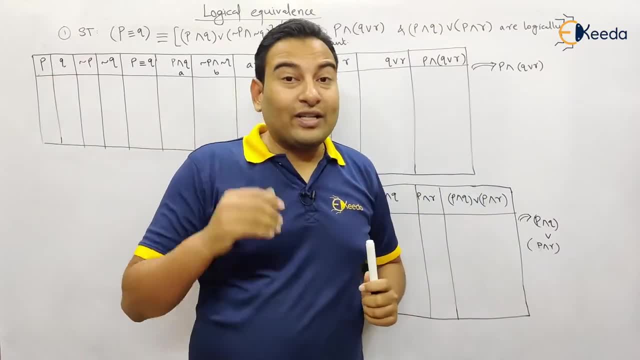 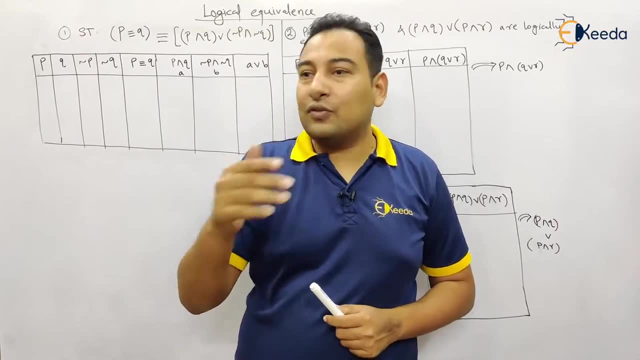 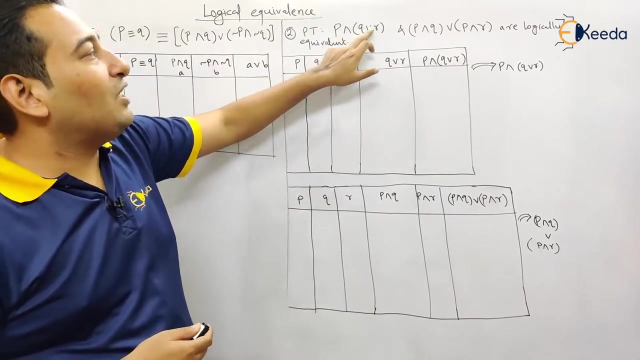 possible. are you clear with this? the first point is how many values we going to consider here, since there are only two and two values, P and Q. therefore, it will be 2 square, that is, four combinations will come here. and what about this particular problem? if you observe this problem, here we have P, Q. 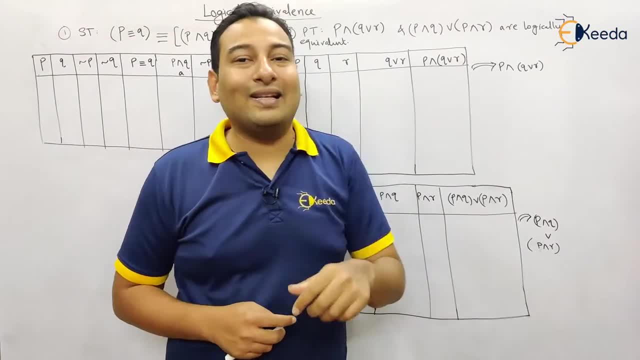 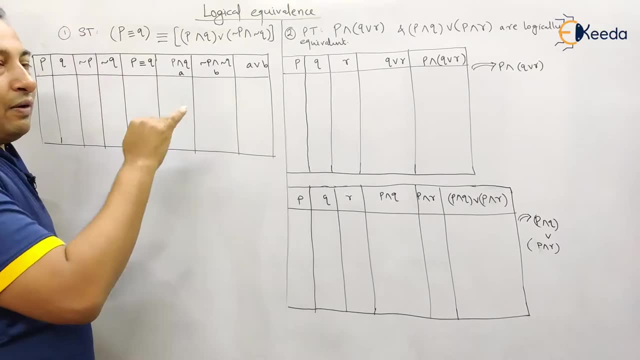 and R. that means three values. therefore 2 cube that will, that is 8 combination will come here. so this is the first point. so let us start now. what are the first points? should we do? what are the four? combination: divide by to half. so first, four means the first two. we'll be true, other two 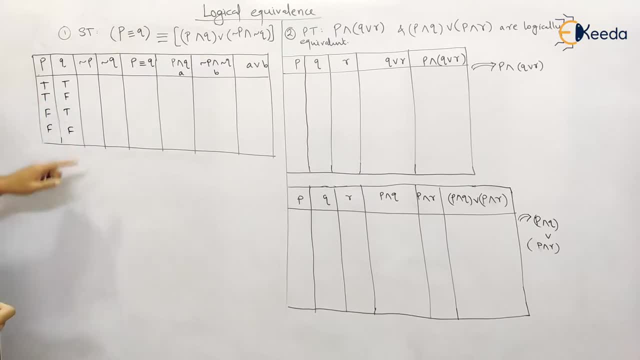 will be false, then it will be alternate true-false. so these are the possibilities. first of all, let us find it out. negation of P: all the truth tables are discussed in the last video and we taking reference from that. so negation of P means just negate it, just oppose it. so to oppose it is false. this is false and the 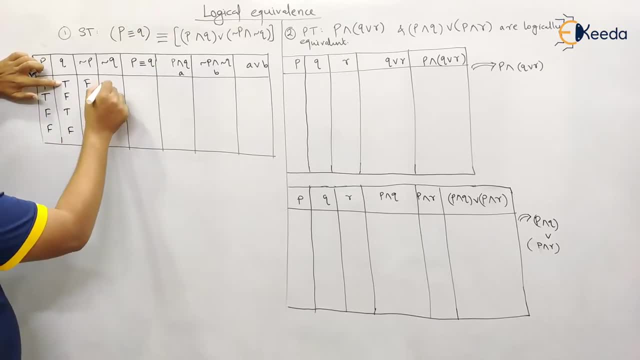 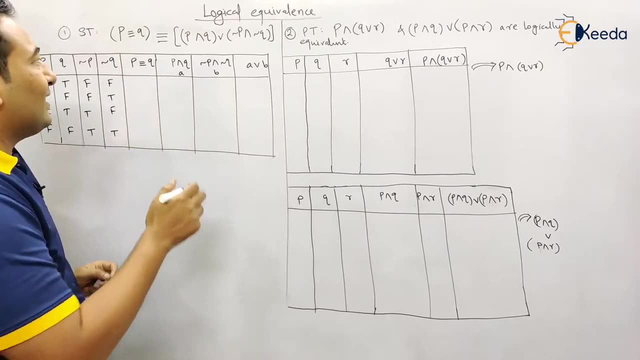 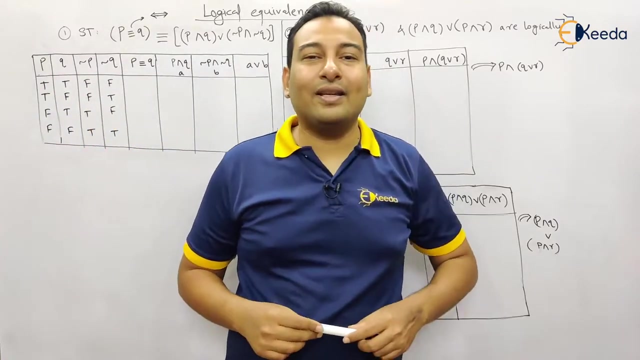 this is true, and this is true. next, negation of q means: this is false, true, false and true. next, what about these three lines? these three lines is basically your by condition. or you can say if and only if. double implication: so it is same, so p double. 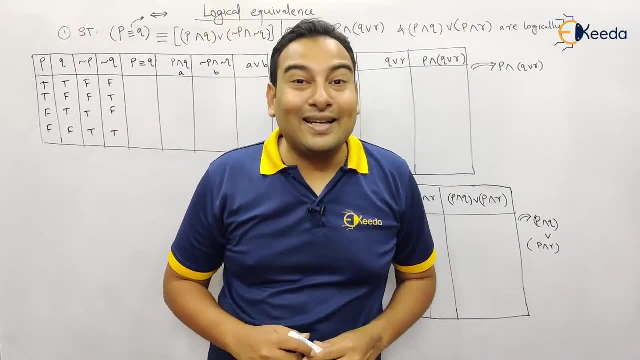 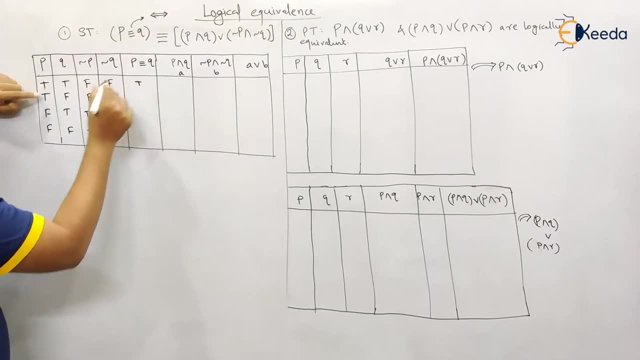 implies q. so remember the truth table, remember the technique: identicals are true. so what do you mean by that? we're going to consider p and q. see, both are true, so it is true. both are false. therefore it is true. identicals are true, they are different, therefore it is false. what next? we want p and q. 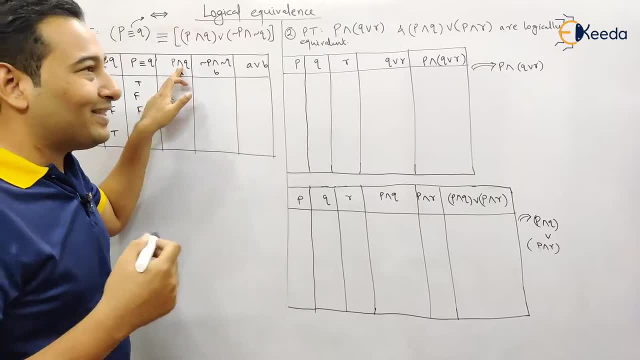 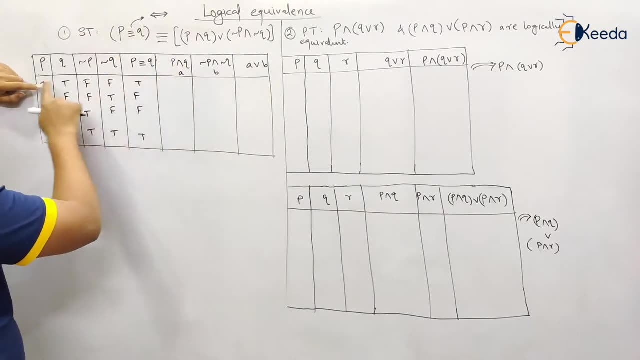 so p and q we want, and, or basically conjunction. what is the truth table? true and true is always true. see here: p and q. so true and true is always true. rest, everything is false. we just need to go step by step and this type of problems are going to be solved. so we're going to go step by step and this type of problems are going to be solved. 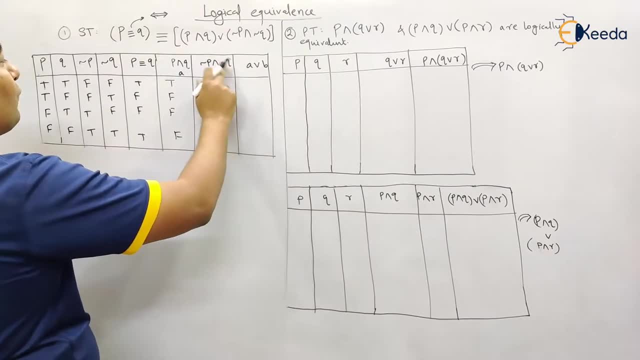 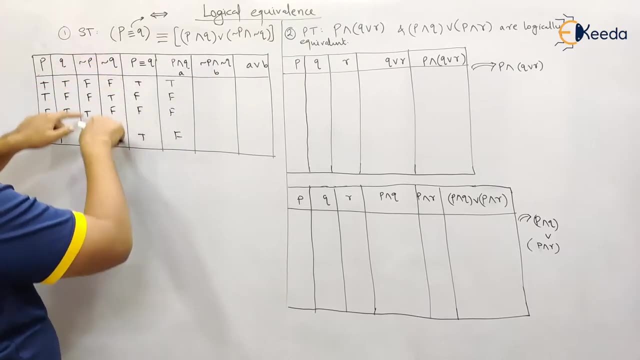 very simple. next, negation of p and negation of q. that means we are talking about between these two, negation of p and negation of q. so i'm going to check proof table or these two columns. so here also in this column, since it is and true and true is always true, see here: true and true is always. 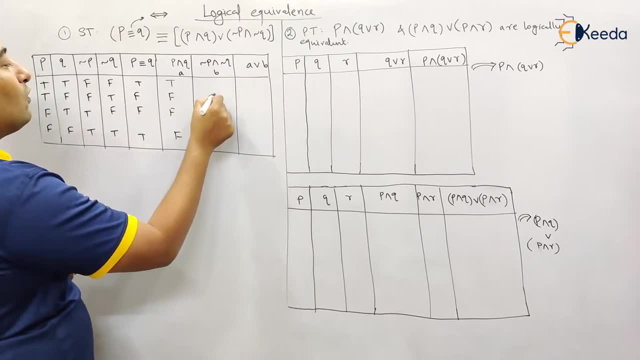 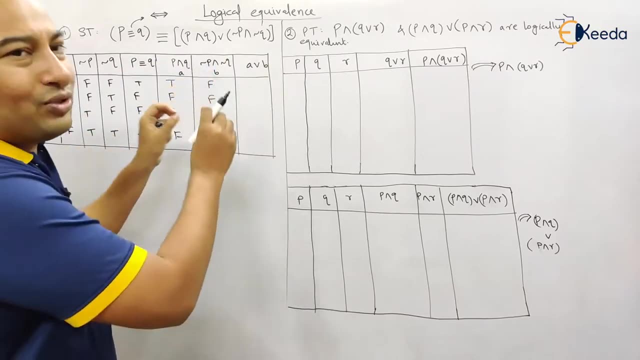 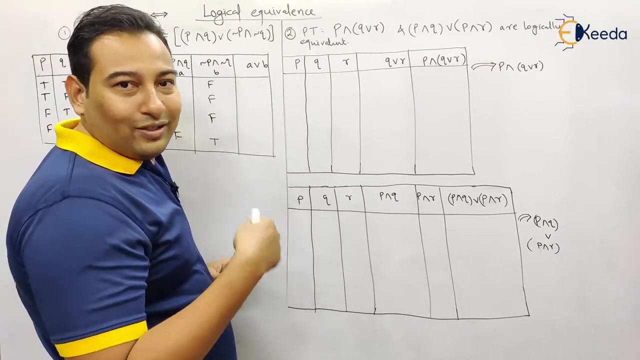 true. rest, everything is false. so this is false, this is false and this is false. and finally, a or b: that means we have named it as a and this is b just to save some space, nothing else. so i need to take or operation between these two and what is or false or false is always so false. 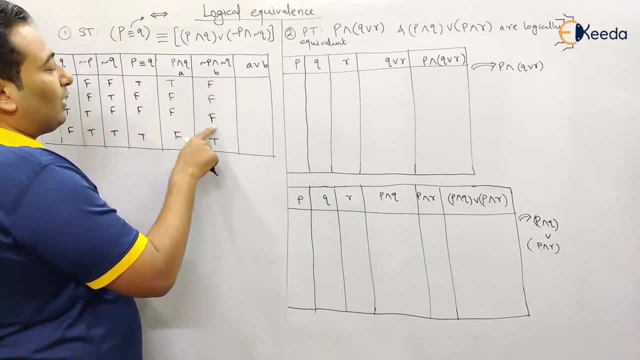 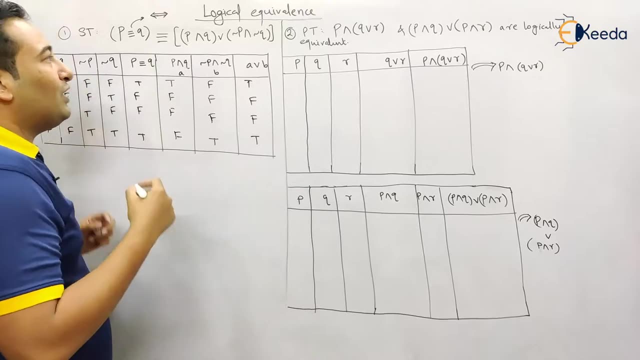 that means if both are false, the result is false. see here: both are false, the result is false. both are false, the result is false. this is true and this is true. now we need to check the logical equivalence. see what is the truth table of this term. see here: this is the truth table. 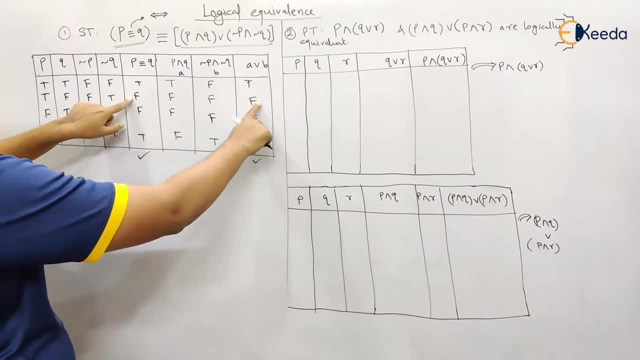 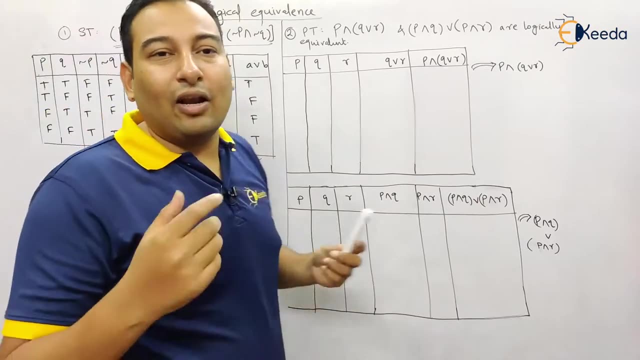 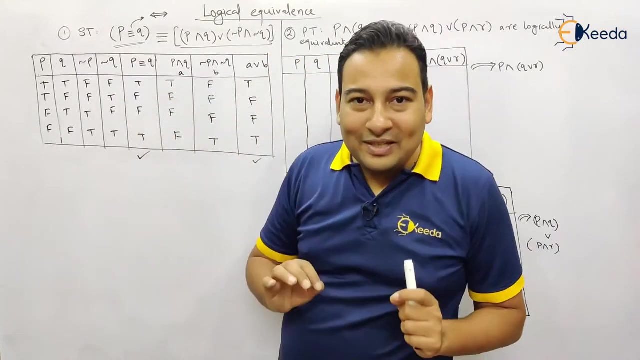 and what about this? this is the true table. see here, they are exactly same. that means if the values in the column are same, then we'll say they are logical equivalent. that's it. is this clear? that means the values in both the column must be same. if they are same, the statements are logically. 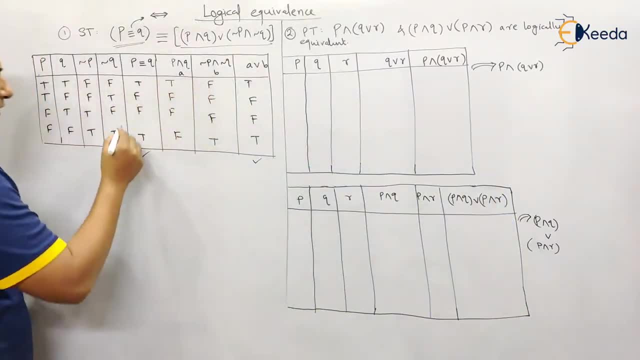 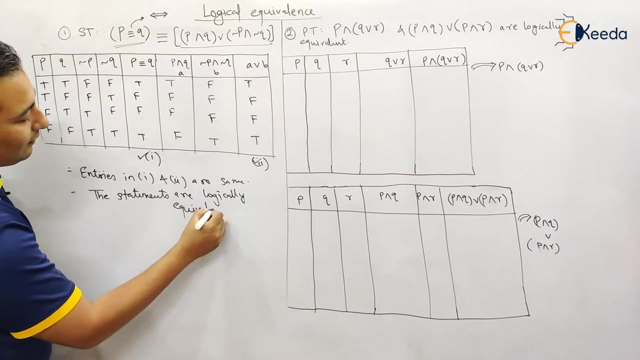 equivalent. that's it. so we can say: let's say this is column number one, let's say column number two. therefore, entries in one and two are same. therefore the statements are logically equivalent. so this is what the proof is. we'll discuss one more example here now, here. 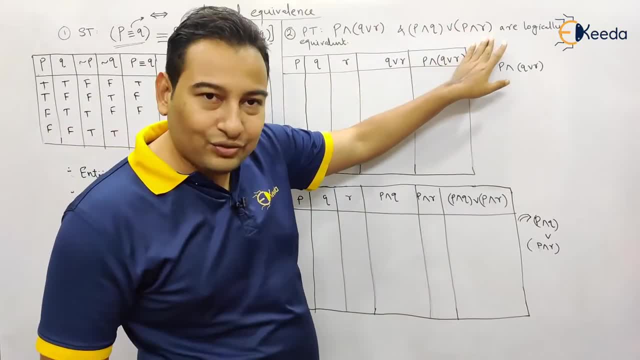 again, there are two statements given. this is your one statement, this is your another statement and we need to prove they are logically equivalent. so we are drawing different truth tables, because if i'll say that i have two statements here and i have two statements here and i have two statements, 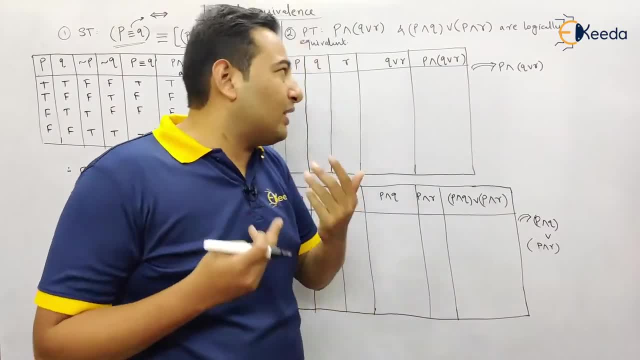 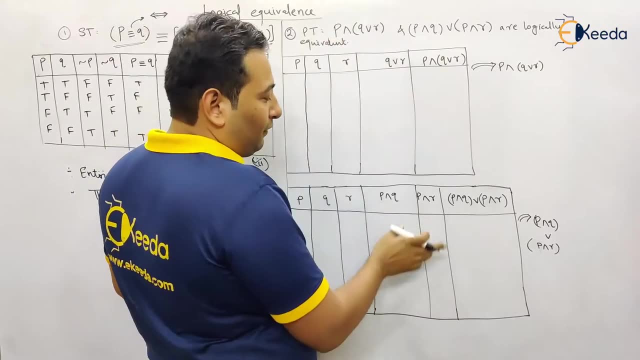 i'll draw in one table. that will be huge and i don't have that much space. therefore, i am drawing it into two different truth tables. so, first of all, we are preparing two table for this statement and after that we are preparing for this statement. now here, if you observe, there are three values: p, q and 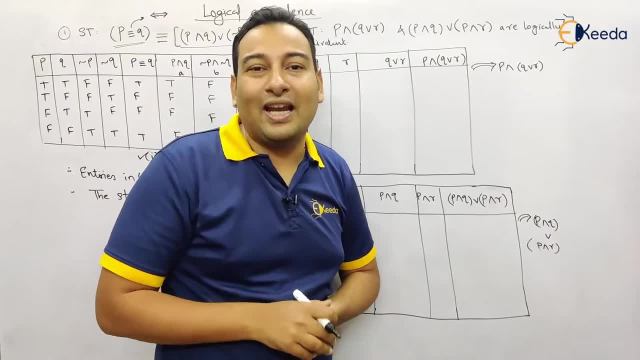 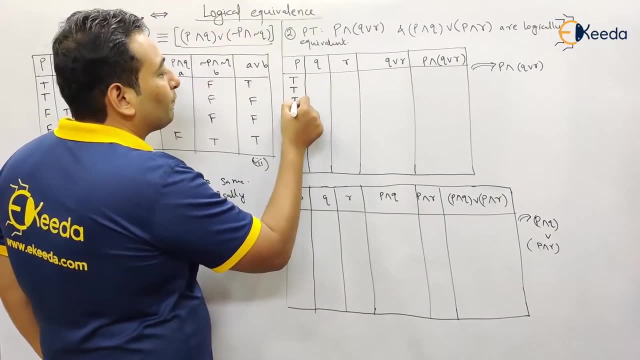 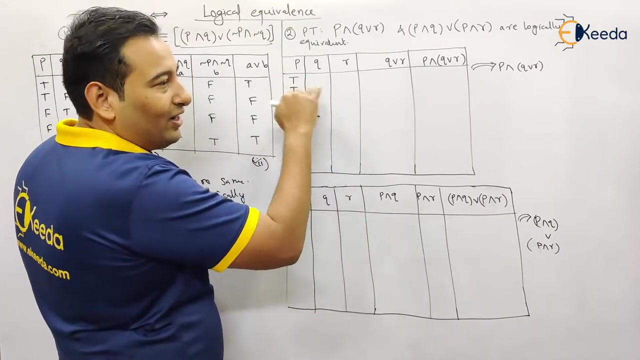 r. so combination will be two cubes. that means there should be eight possibilities. now what is the first step? divide eight into two. that means four. so it will be four true, and after that four false. what next? four, two, four, false. then again divide two by divide by two. that means two true, two false. 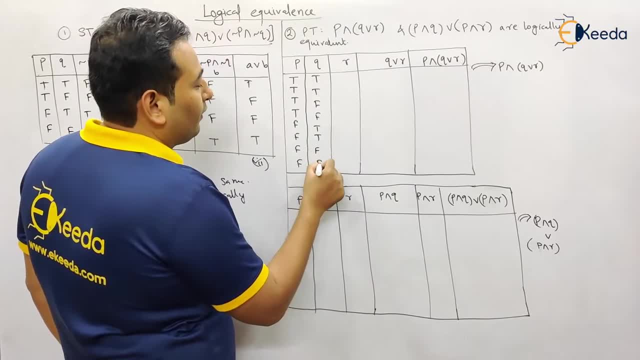 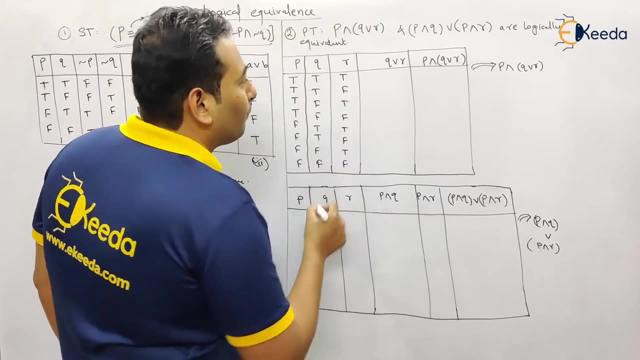 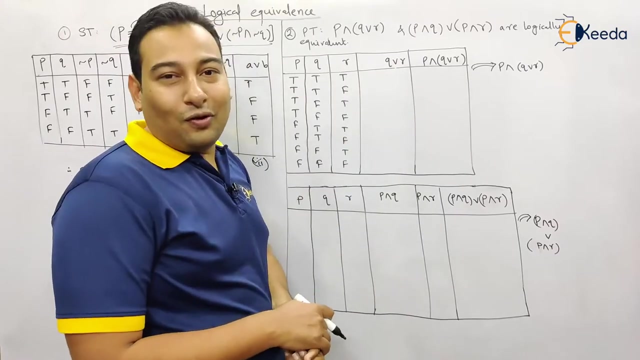 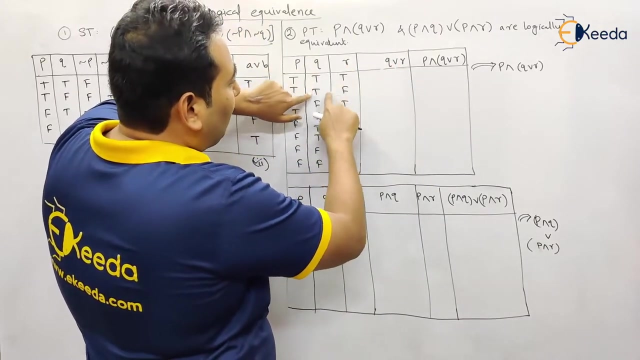 two true and two false and finally alternate true- false. next we need to find it out: q or r. so this is what your disjunction or, or means, what false or false is always a false and we'll will see in q or r table. so if both are false, then it is false. let me draw this. 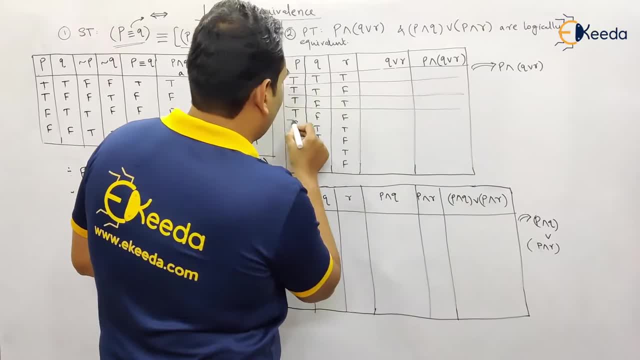 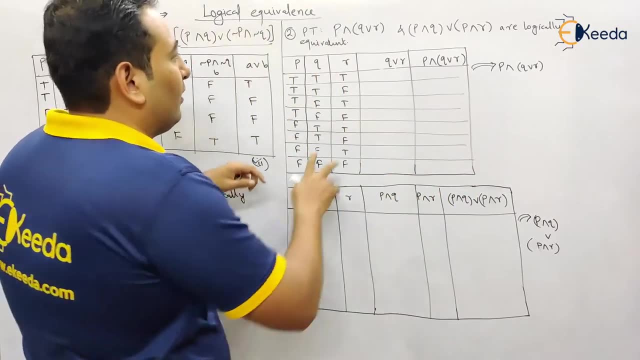 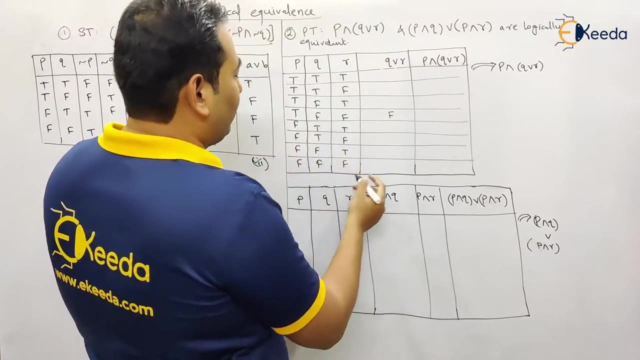 otherwise it will get mixed up. so i don't want any confusion now it is clear. now let's check q or r, both false. i'm looking out for both false. false or false is always false. rest of see here one more: false or false is always false. rest everything. 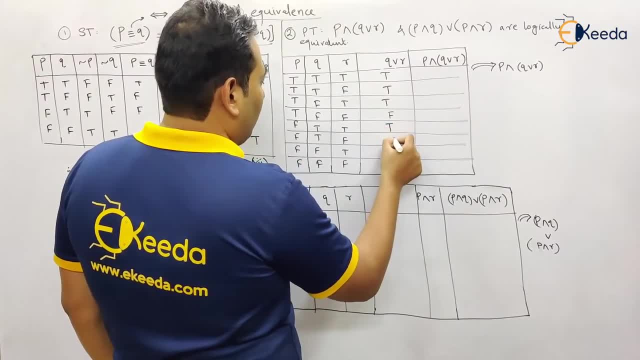 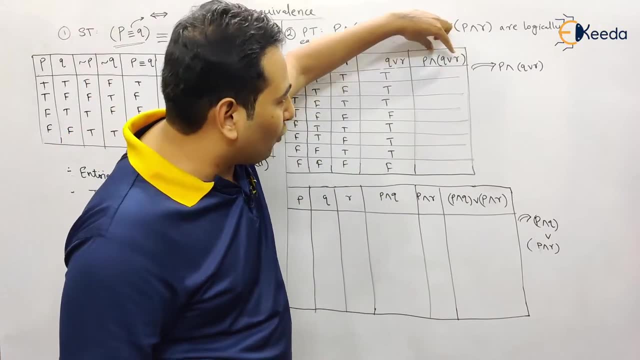 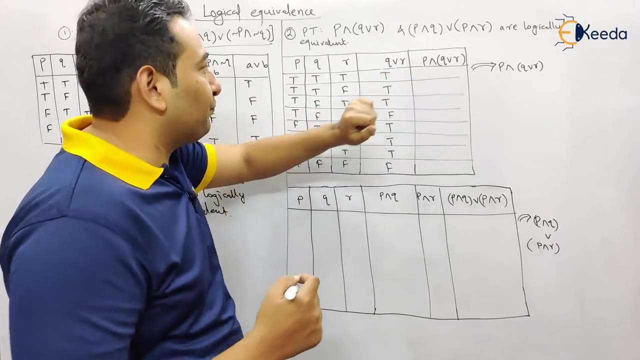 is true. so this is true, this is true, this is true, true, true and true. what next? p and q or r? so q or r, we already found out. we just need to take q or r and p conjunction. that means, and so basically we are referring to p and this particular table, this particular column. so we are looking out for. 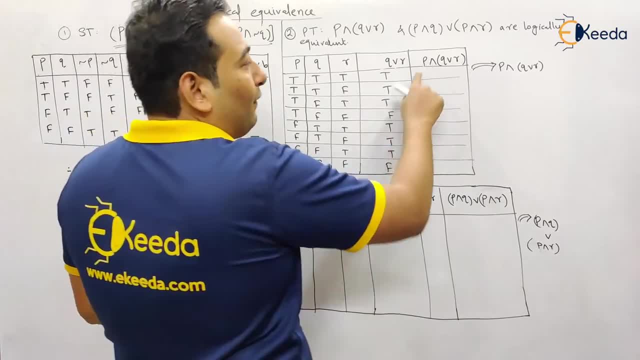 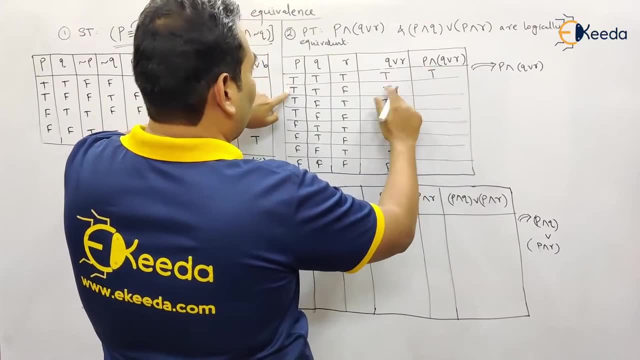 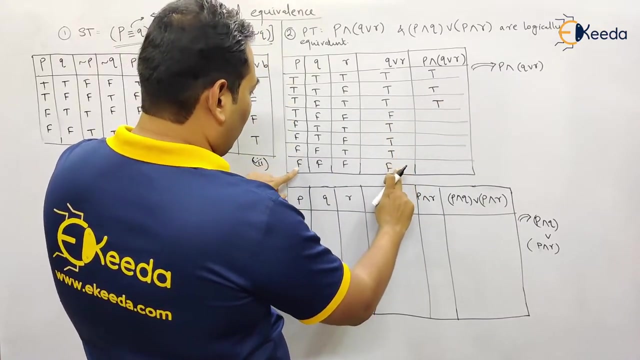 these two columns, p and this particular column, and in between we have. and so what do you mean by and true and true is always true. so let us check, see here: both are true, it's true. both are true, again true, both are true, again true. true and true is always true. rest, everything is false. so there are three occasions. 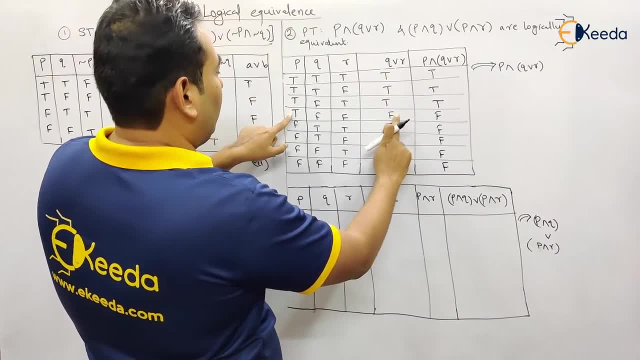 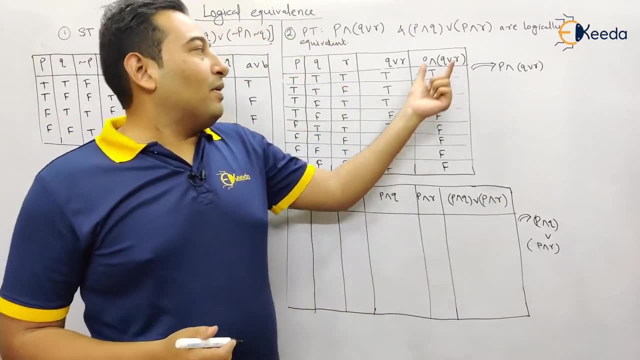 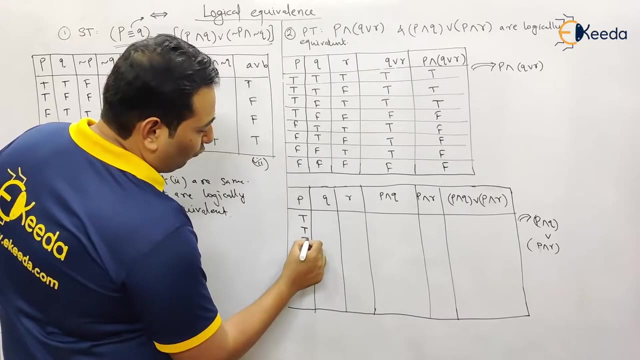 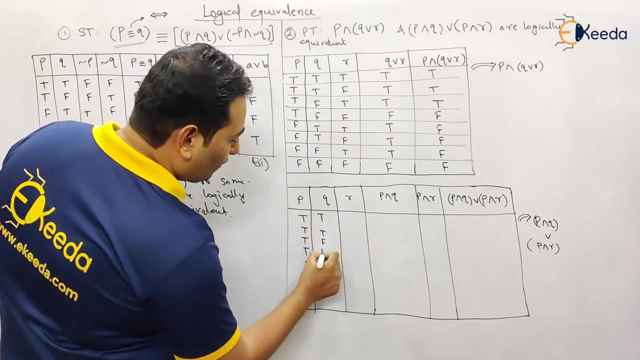 we are getting both true. see here here: one true, one false. then we are not getting both true. so this is your truth table for this particular statement. now let us check root table for the second statement. again same thing for true, for false. then what? two true, two false. two true, two false. then true, false. 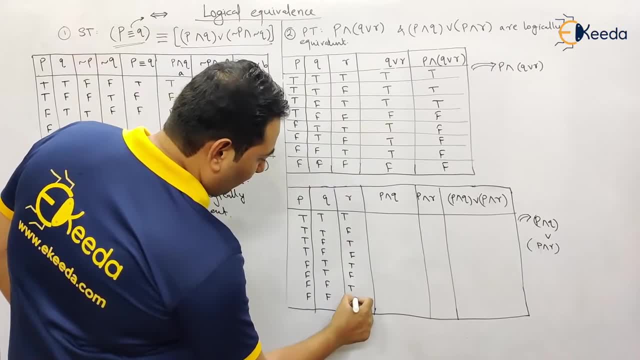 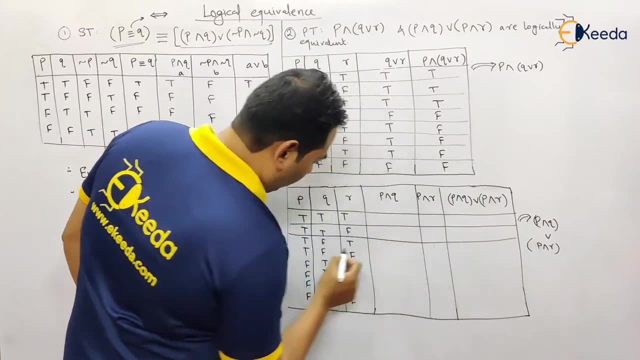 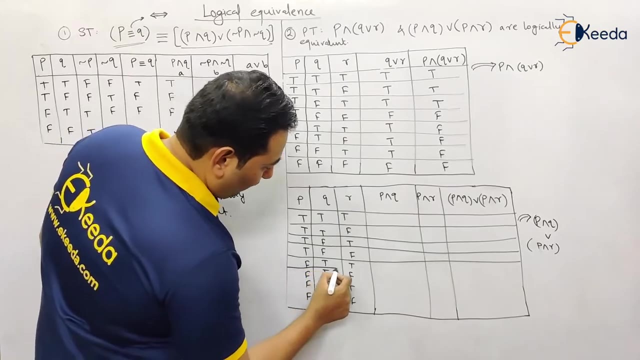 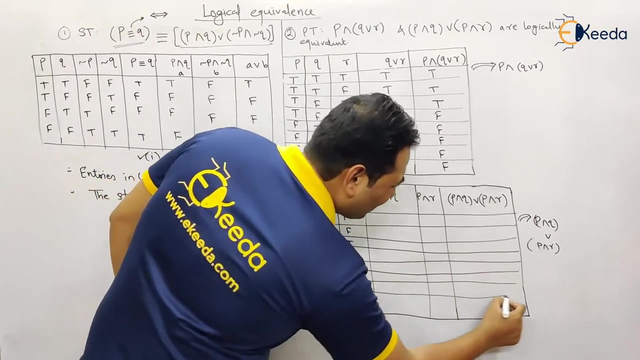 true, false, true, false and true and false again. let me separate so that there should not be any confusion, so that there should not be any confusion: one mess up here and there, the whole table will go wrong. so therefore, you should be very careful while drawing this table. this is very 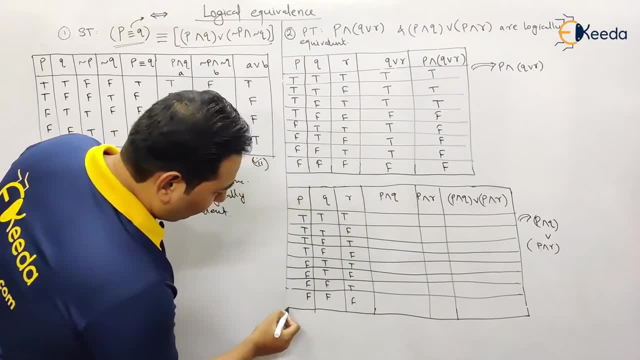 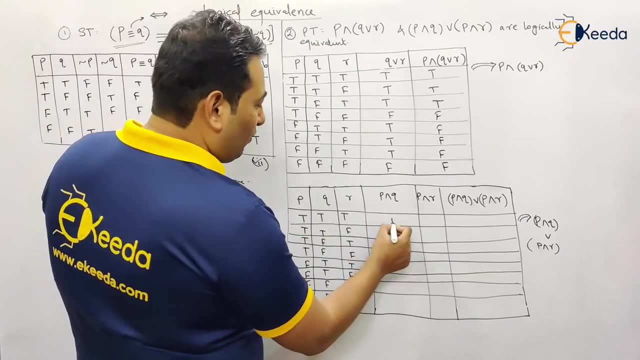 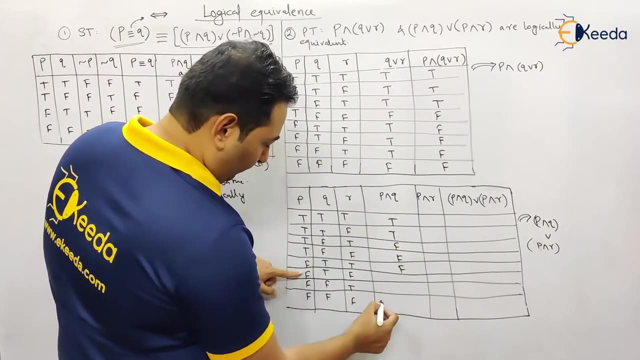 simple thing, but yes, you should be careful. p and q, so we need to take p and q. pro and pro is always true. see here: pro and pro is always true, true and true is always true. this is false. this is false. this is false, again, false, again, false and finally false. so there are only 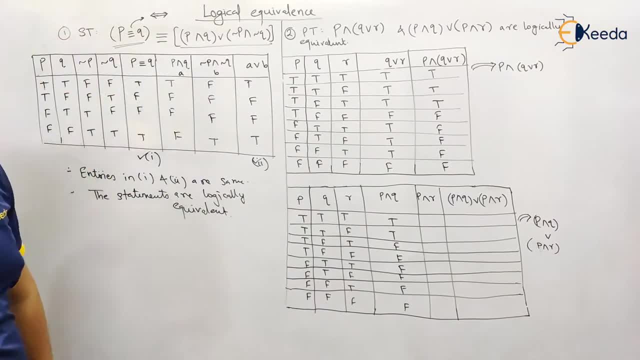 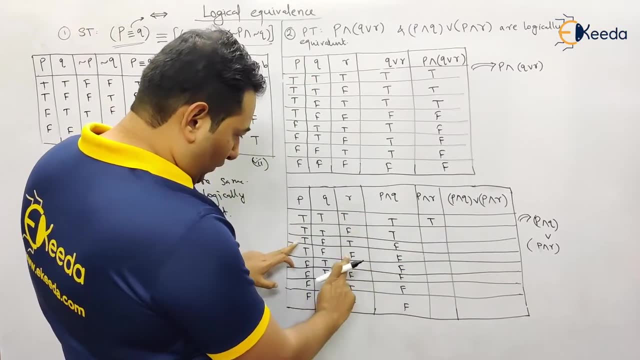 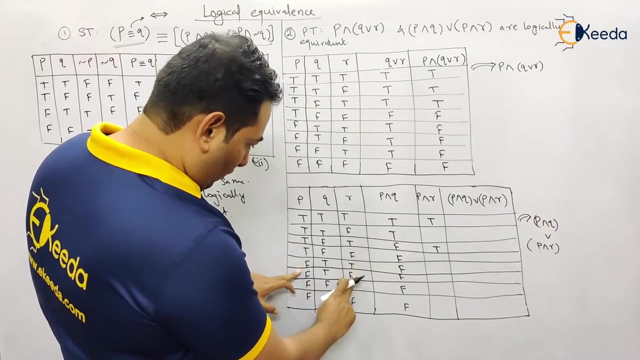 two vocation, in which both are true, rest everywhere. it is false. what next? r p and r? we need to check p and r. so this is true, where this is. for again, this is true. what next? this is false, false, that's it. rest everywhere. it is false.